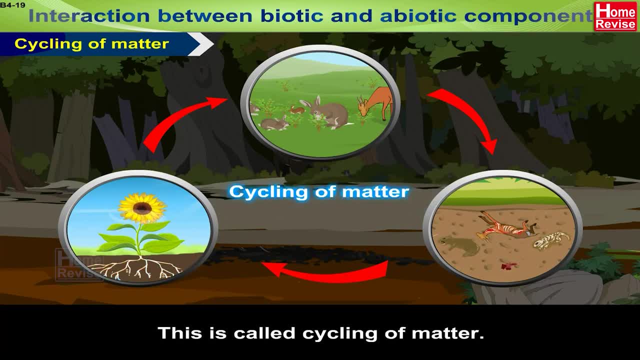 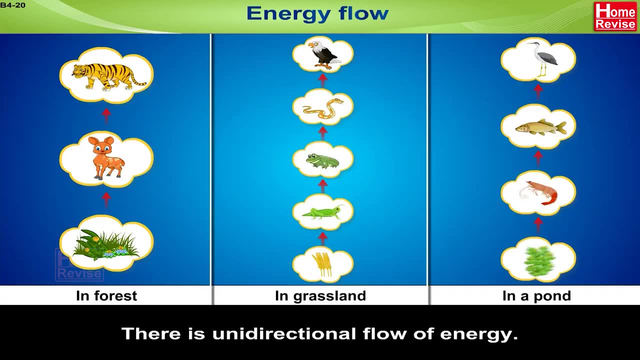 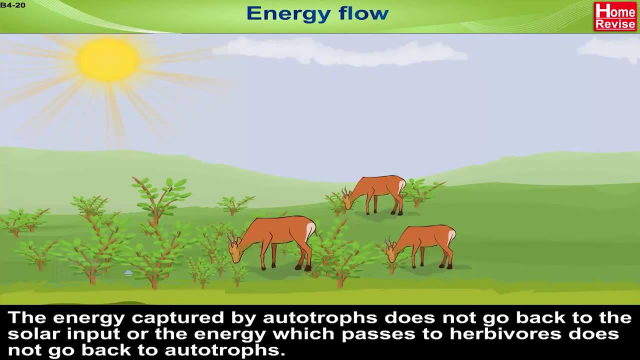 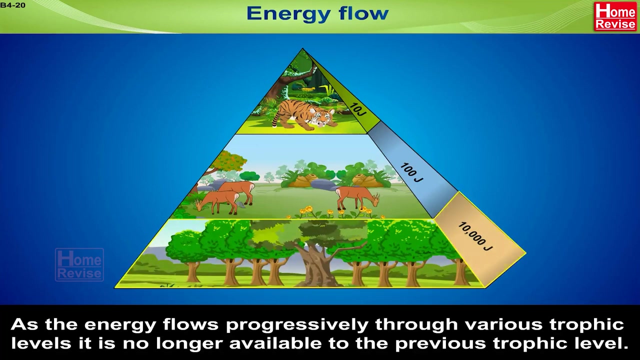 This is called cycling of matter Energy flow. There is unidirectional flow of energy. The energy captured by oil and gas is then absorbed by the producers. The energy that is absorbed by ototrophs does not go back to the solar input or the 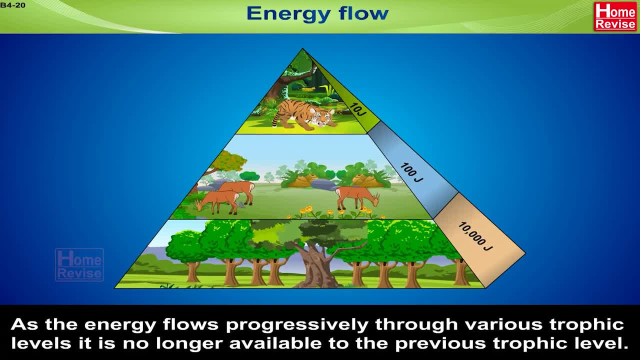 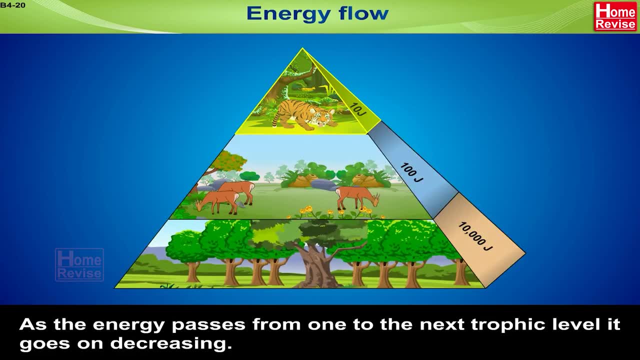 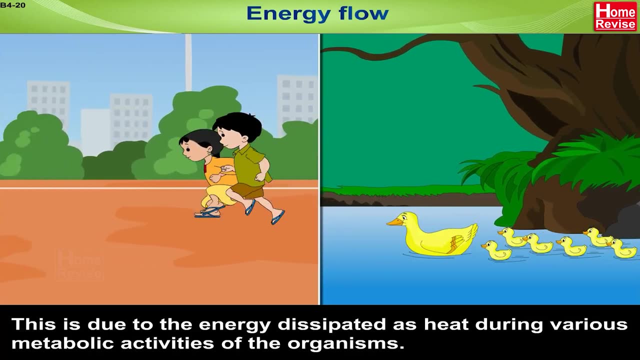 energy which passes to herbivores does not go back to ototrophs. As the energy flows progressively through various trophic levels, it is no longer available. This is due to the energy dissipated as heat during various metabolic activities of the organisms. 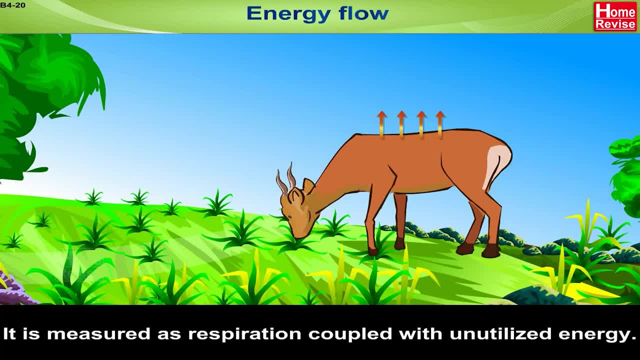 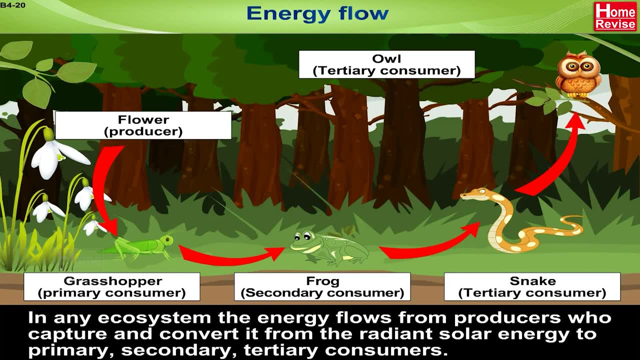 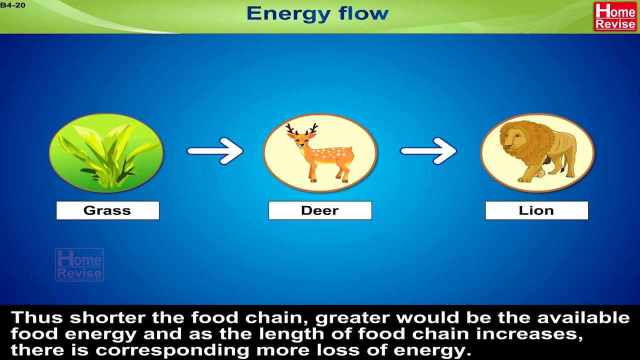 It is measured as respiration coupled with unutilized energy. In any ecosystem, the energy flows from producers who capture and convert it from the radiant solar energy to primary, secondary, tertiary consumers. Thus, shorter the food chain, greater would be the available food energy and as the length, 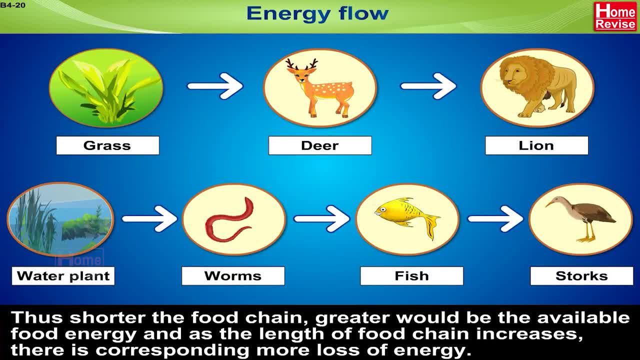 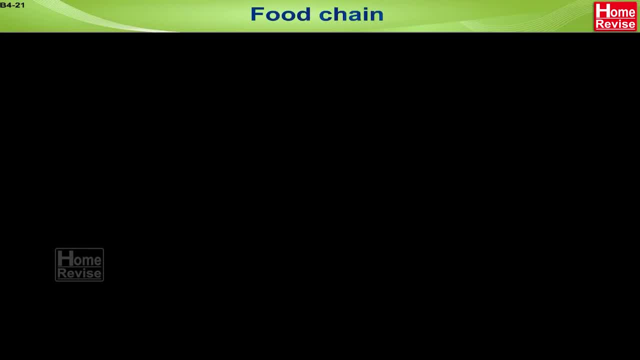 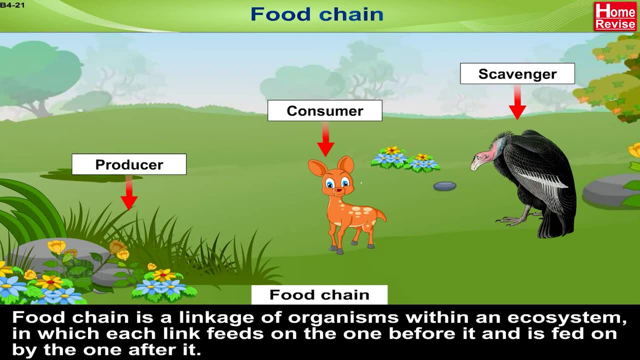 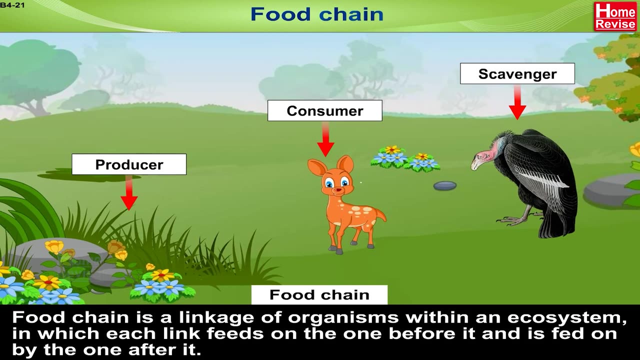 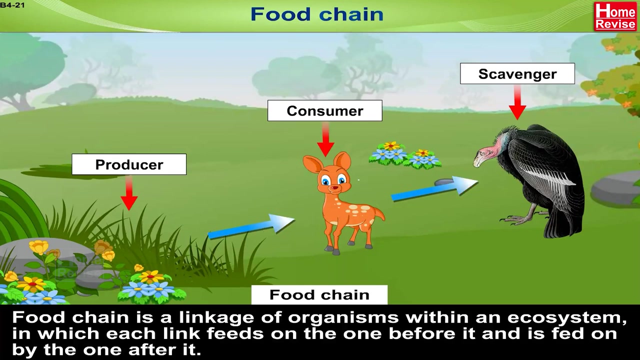 of food chain increases, there is corresponding more loss of energy Food Chains. Do you know what is a food chain? Well, food chain is a linkage of organisms within an ecosystem in which each link feeds on the one before it and is fed on by the one after it. 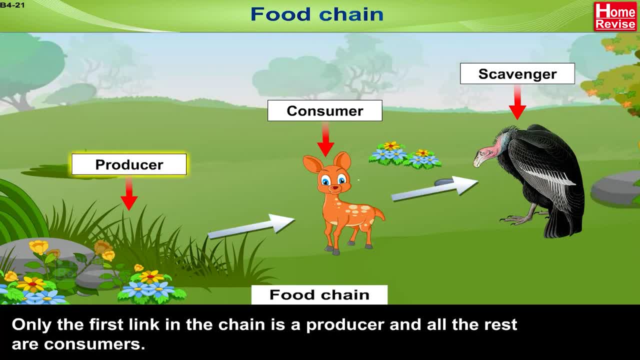 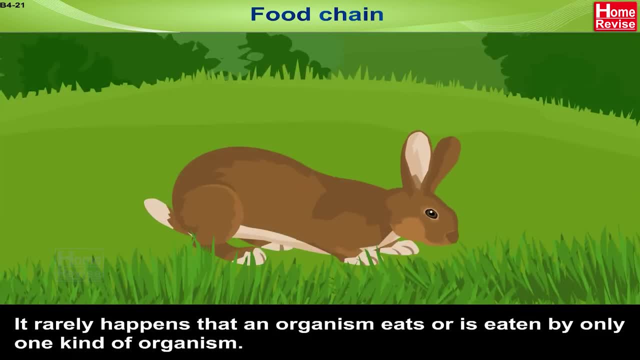 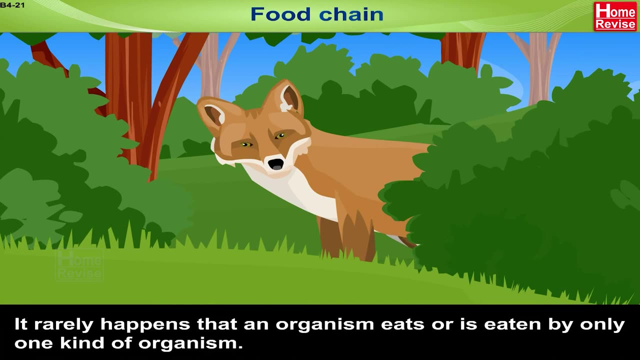 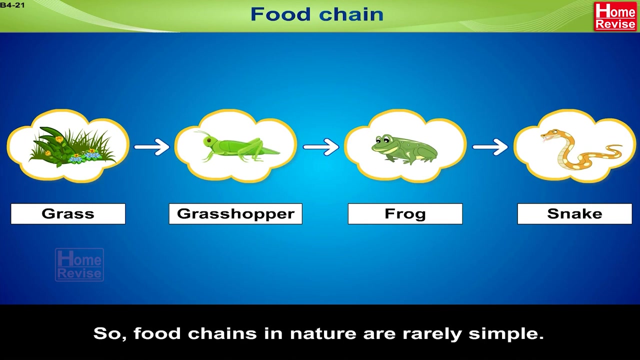 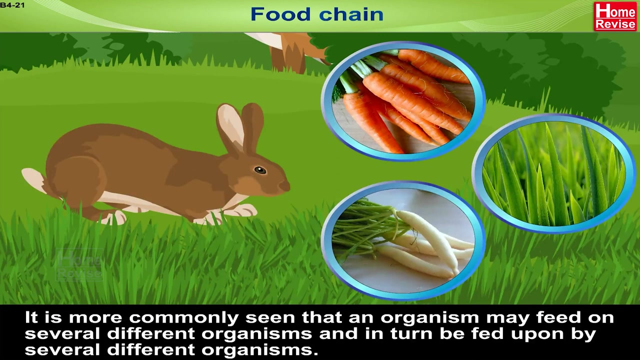 Only the first link in the chain is a producer and all the rest are consumers. It rarely happens that an organism eats or is eaten by only one kind of an organism, So food chains in nature are rarely simple. It is more commonly seen that an organism may feed on several different organisms and 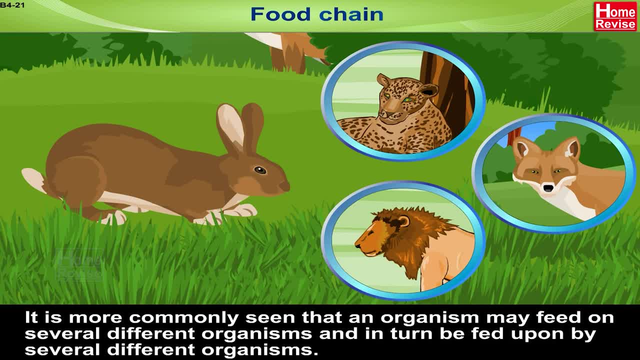 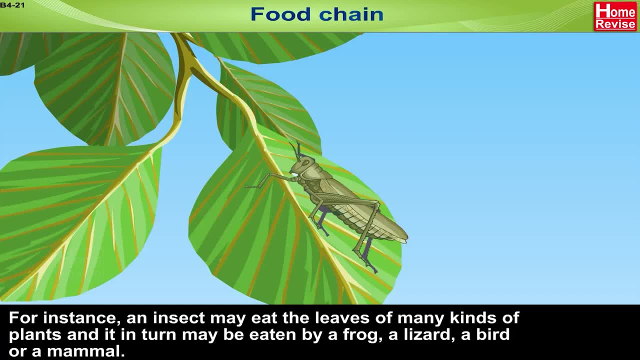 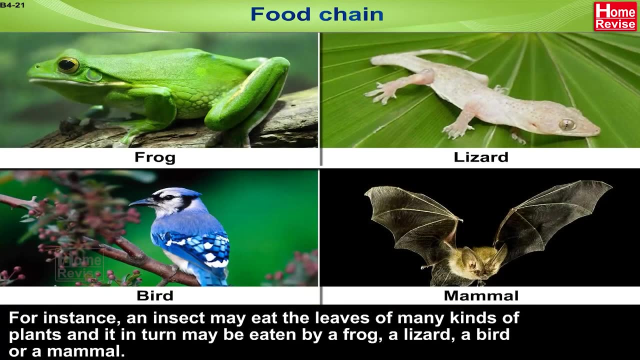 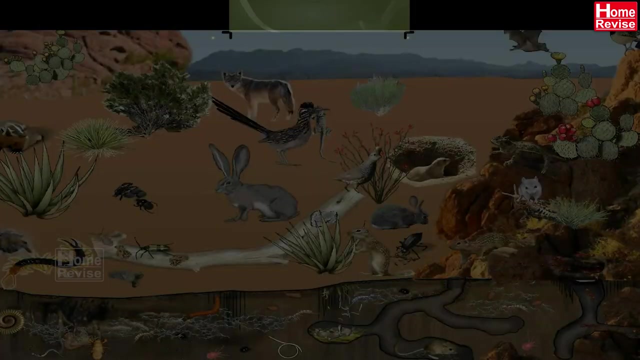 in turn be fed upon by several different organisms. What is a food chain? For instance, an insect may eat the leaves of many kinds of plants, and it in turn may be eaten by a frog or a lizard, a bird or a mammal. 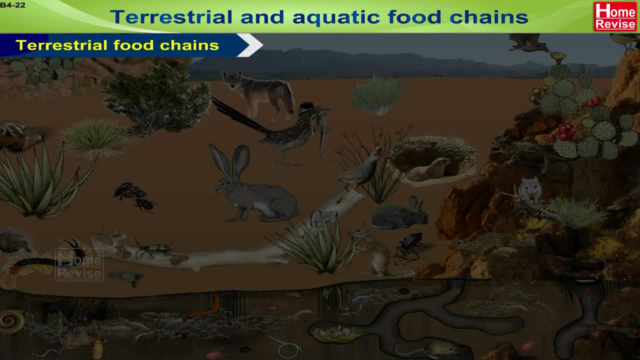 Terrestrial and Aquatic Food Chains. Terrestrial Food Chains: A food chain found in a grassland or a forest is a food chain. Terrestrial Food Chains: A food chain found in a grassland or a forest is a food chain. A food chain is a food chain. 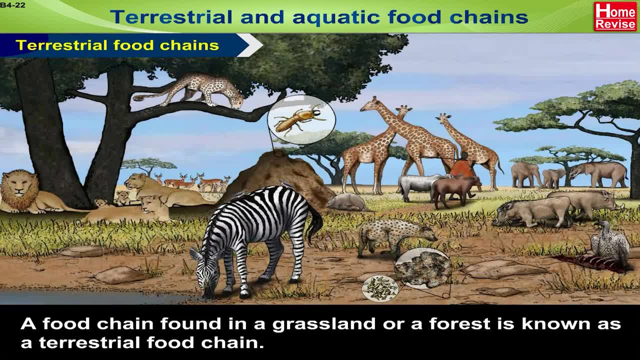 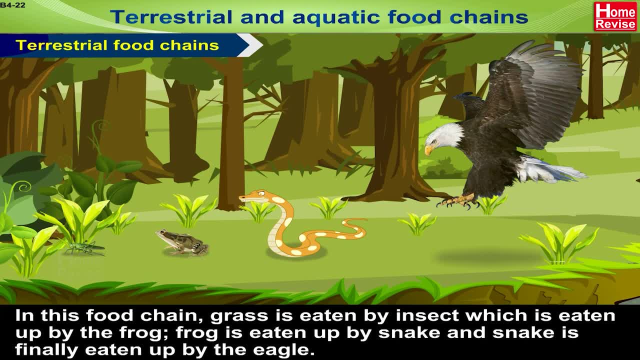 A food chain is a food chain is known as a terrestrial food chain. The figure shows such a food chain. In this food chain, grass is eaten by insect, which is eaten up by the frog, Frog is eaten up by snake, and snake is finally eaten up by the eagle. 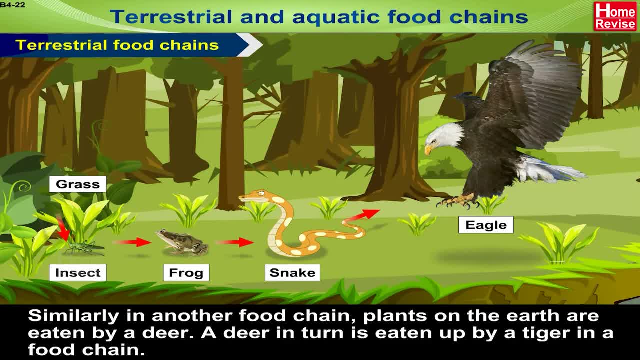 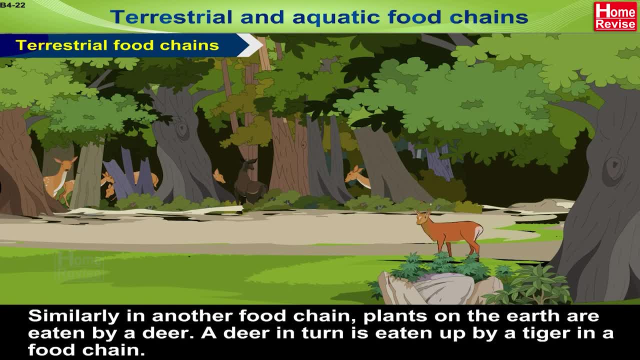 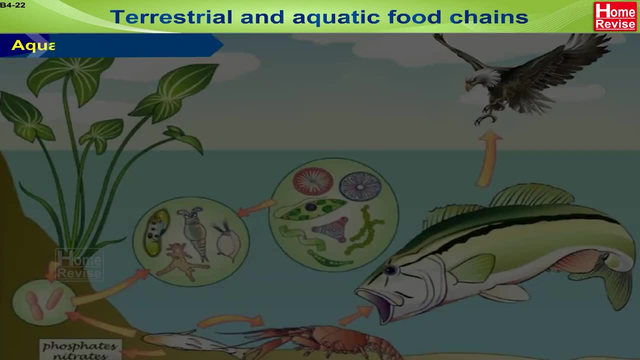 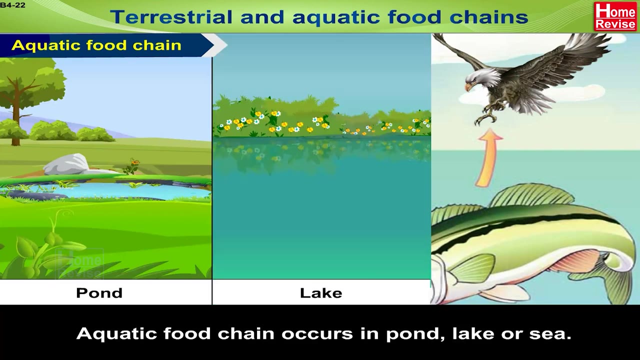 Similarly in another food chain, plants on the earth are eaten by a deer. A deer in turn is eaten up by a tiger in a food chain- Aquatic food chain. Aquatic food chain occurs in pond lake or sea, In it weeds. 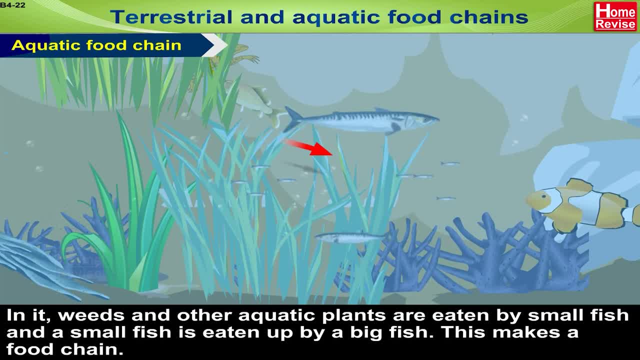 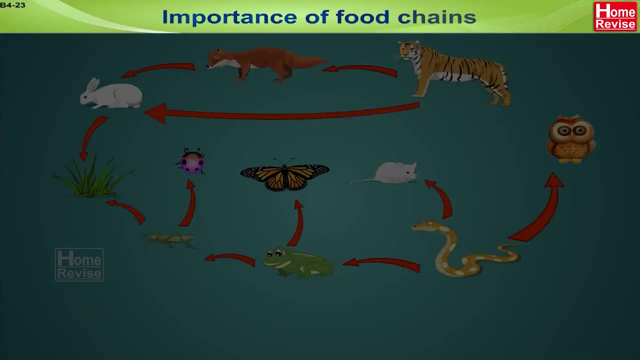 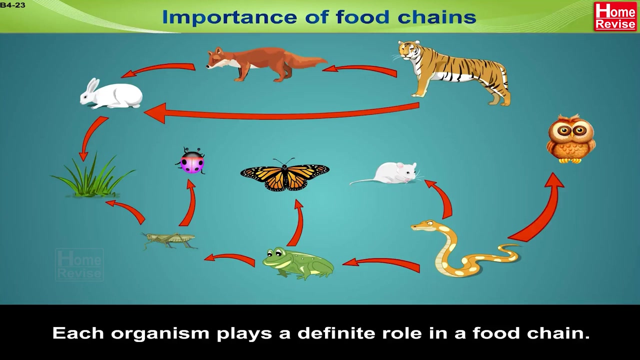 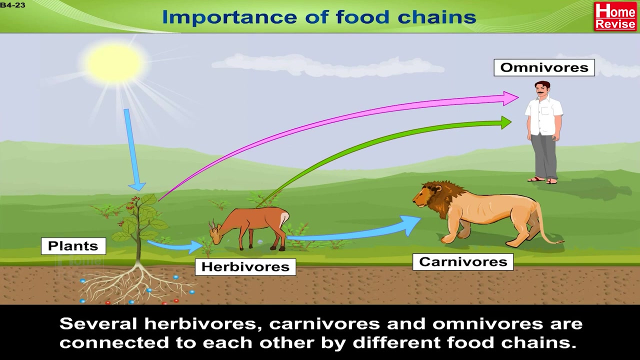 and other aquatic plants are eaten by small fish, and a small fish is eaten up by a big fish. This makes a food chain. Importance of food chains. Each organism plays a definite role in a food chain. Several herbivores, carnivores and omnivores are connected to each other by different food chains. 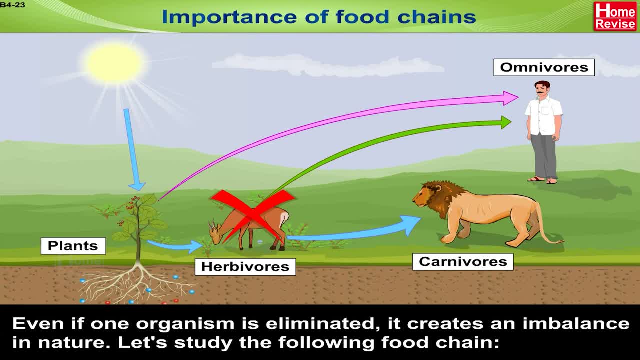 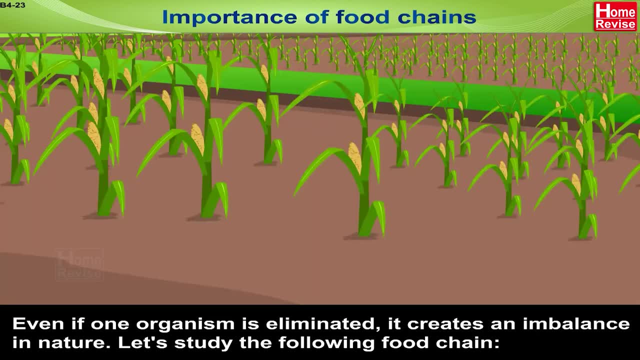 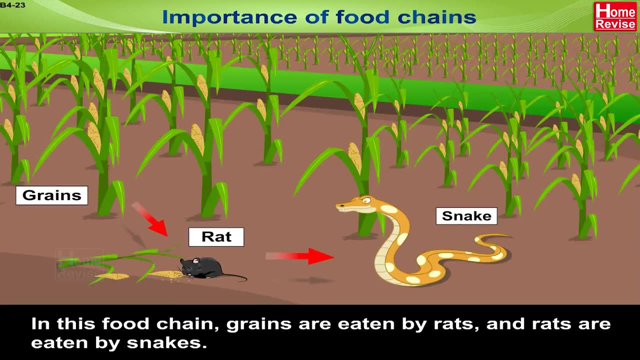 Even if one organism is eliminated, it creates an imbalance in nature. Let's study the following food chain. In this food chain, grains are eaten by rats and rats are eaten by snakes. Somehow, if all the snakes are eliminated from the food chain, 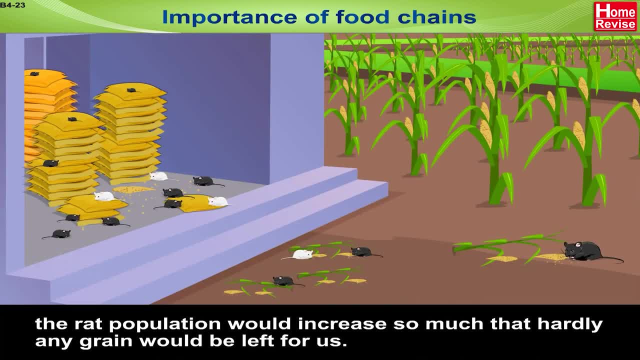 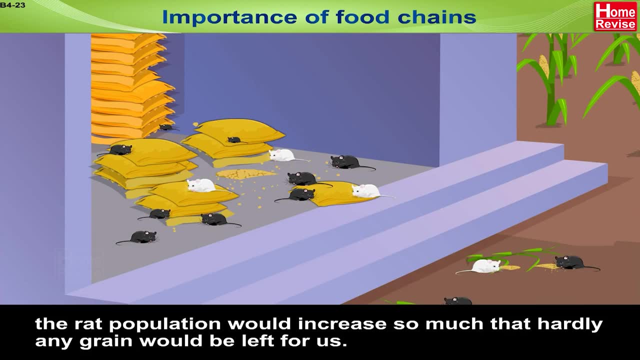 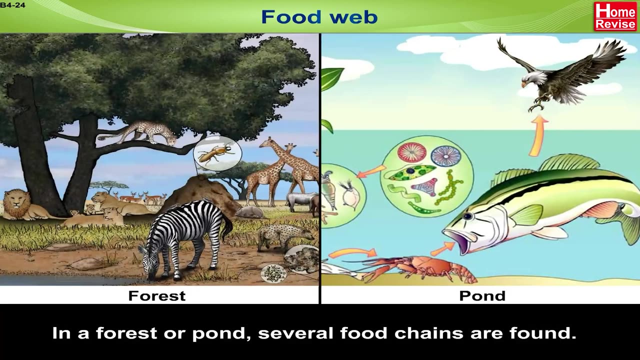 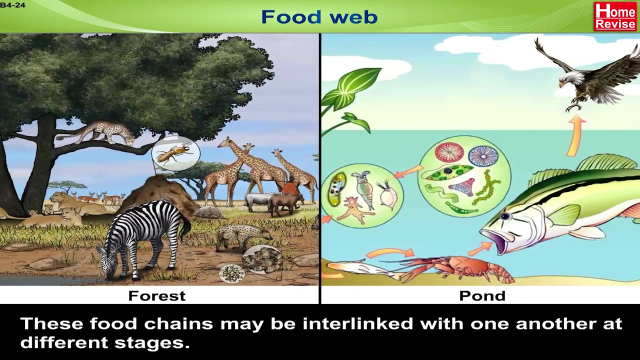 chain. the rat population would increase so much that hardly any grain would be left for us. That's something to think about. Food Web: In a forest or pond several food chains are found. These food chains may be interlinked with one another at different stages. 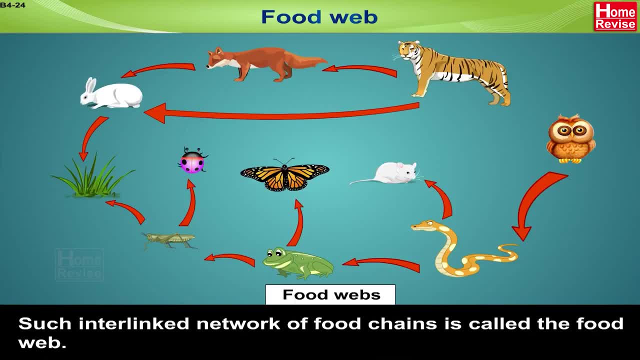 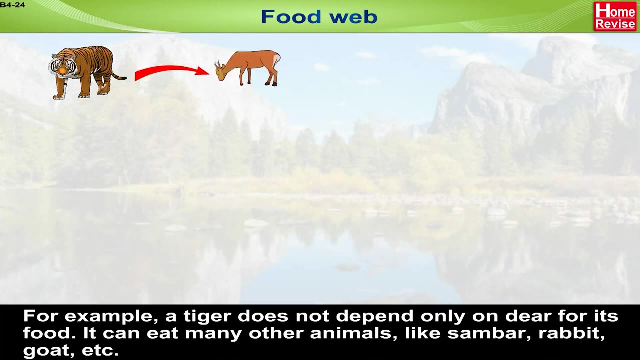 Such interlinked network of food chains is called the food web. In a food web, most consumers have more than one source of food. For example, a tiger does not depend only on deer for its food. It can eat many other animals, like some animals. 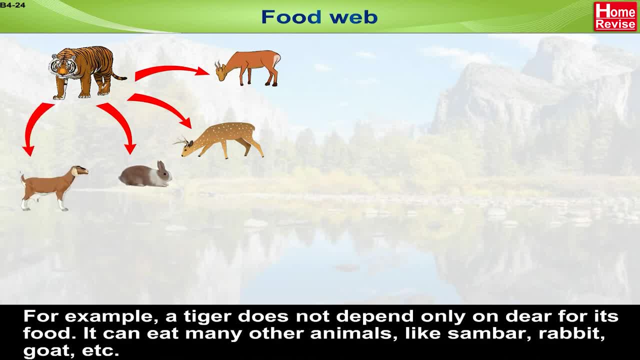 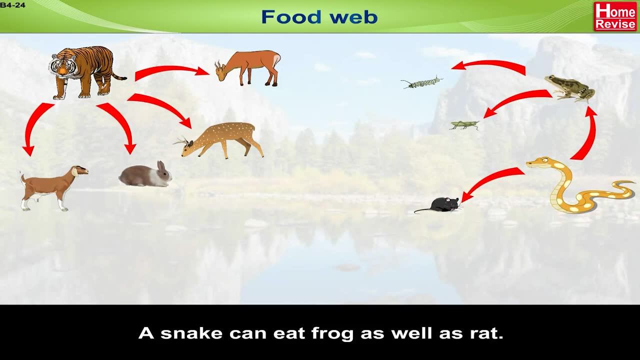 For example, it can eat a cucumber, rabbit, goat, etc. Similarly, a frog can eat caterpillars or grasshoppers. A snake can eat frog as well as rat. Rats are also eaten by hawks. Likewise, grass is not only eaten by a deer, it is also the food of cow, buffalo. 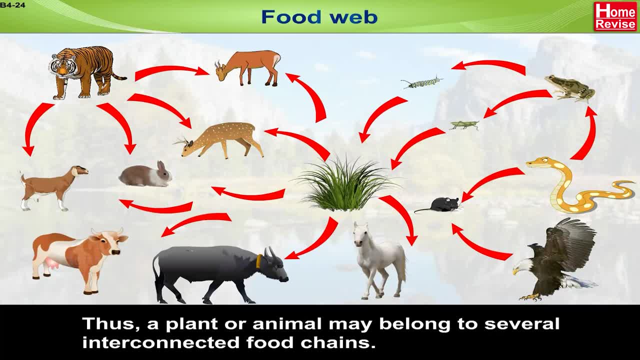 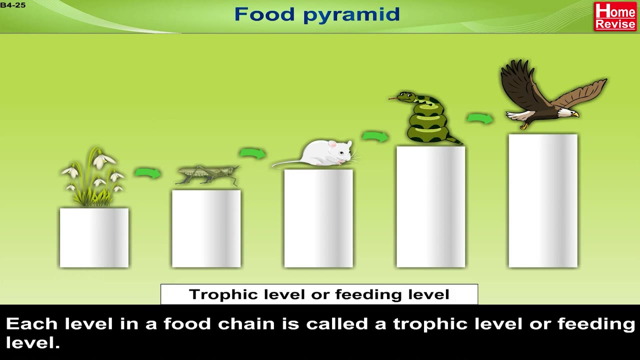 and horse. Thus, a plant or animal may belong to several interlinked food chains. This interlinked network of food chains gives rise to a food web Food Pyramid. Each level in a food chain is called a trophic level or feeding level. 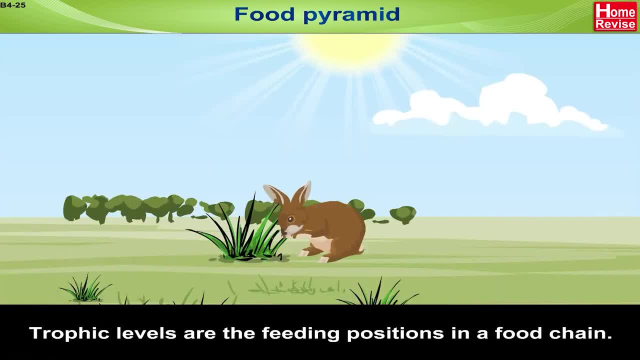 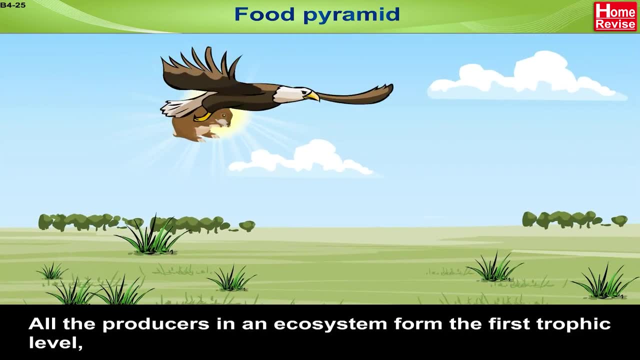 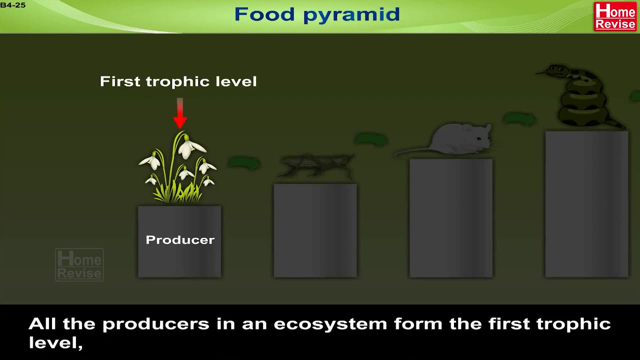 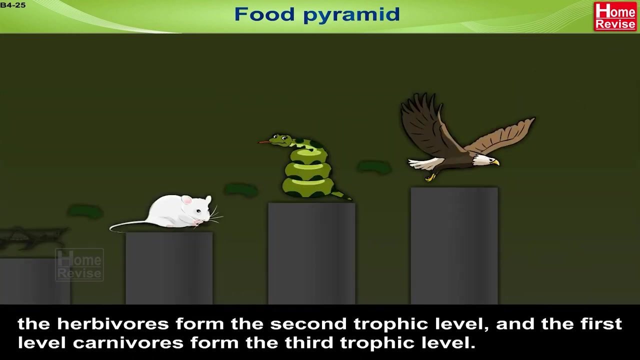 Now trophic level. What is a trophic level? Trophic levels are the feeding positions in a food chain. All the producers in an ecosystem form the first trophic level. The herbivores form the second trophic level. 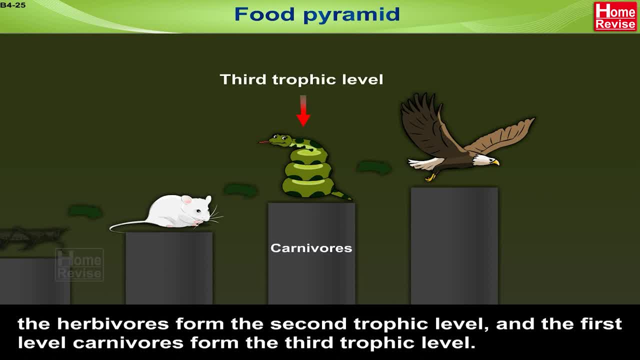 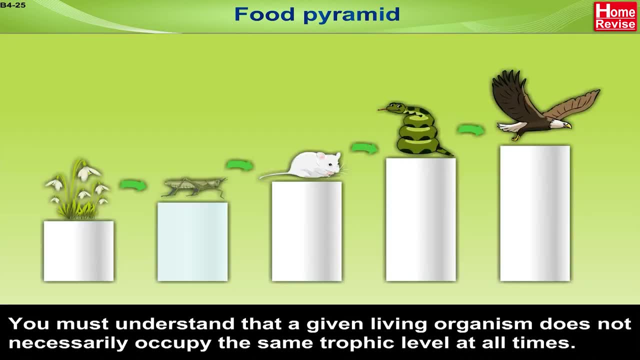 And the first level. carnivores form the third trophic level. You must understand That a given living organism does not necessarily occupy the same trophic level at all times. Say, for example, grass ie producers is the first trophic level. 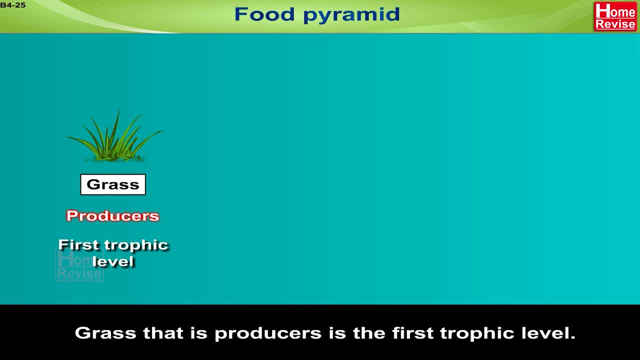 It gets eaten by rabbit herbivores. second trophic level. The rabbit ie producers is the second trophic level. The rabbit ie producers is the first trophic level. The rabbit ie producers is the second trophic level. 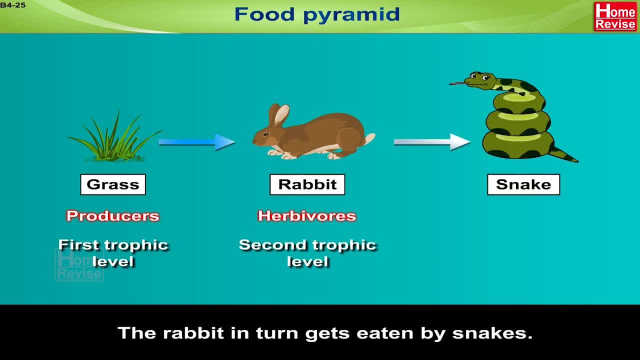 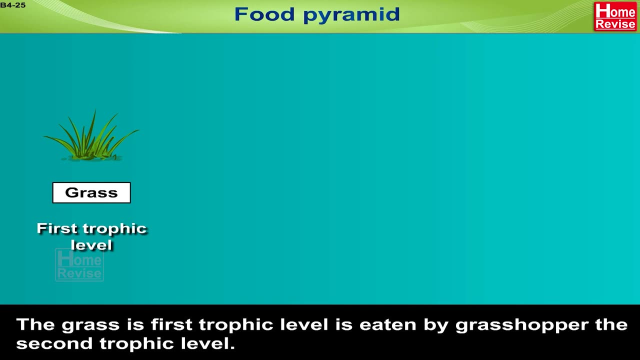 The rabbit in turn gets eaten by snakes, ie carnivores, the third trophic level. In another example, Grass- the first trophic level- is eaten by grasshopper. the second trophic level- Grasshopper- is eaten by frog. 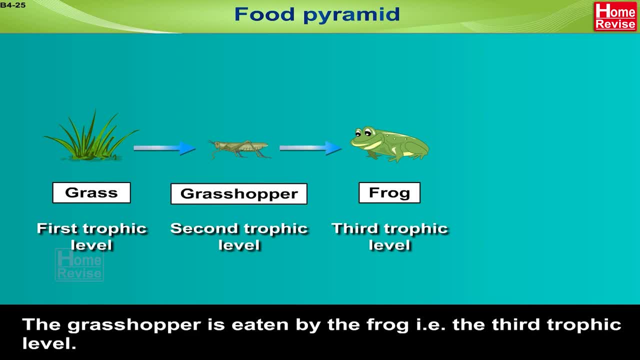 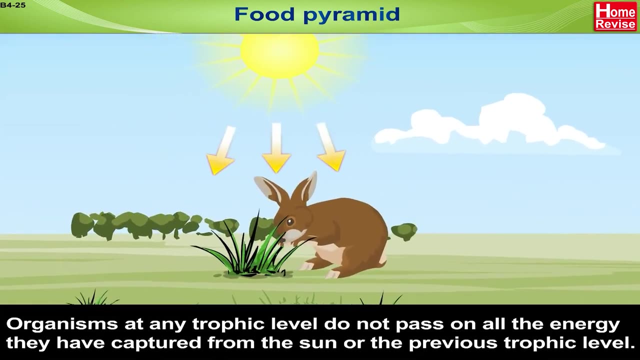 Grasshopper is eaten by frog- That is the third trophic level- and the frog, in turn, is eaten by the snake, the fourth trophic level. Organisms at any trophic level do not pass on all the energy that they have captured. 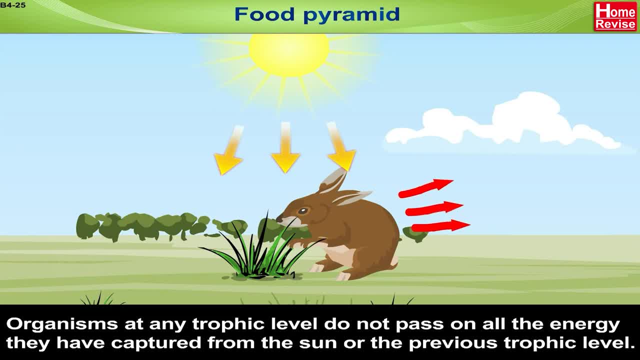 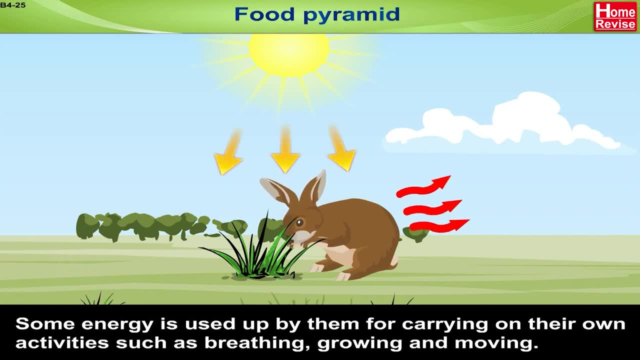 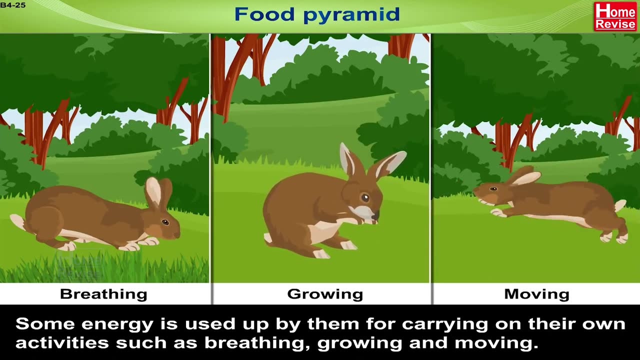 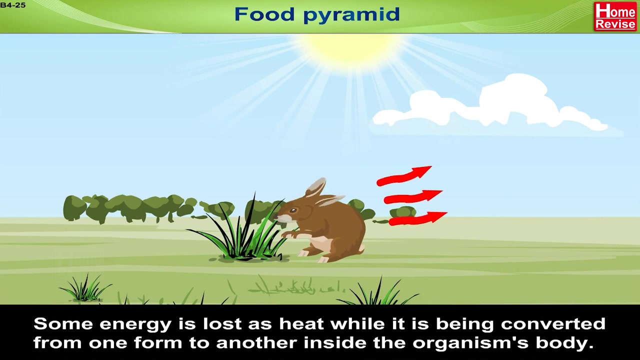 from the sun or the previous trophic level. Naturally, some energy is used up by them for carrying on their own activities, such as breathing, crowing and moving. Some energy is lost as heat while it is being converted from one form to another inside. 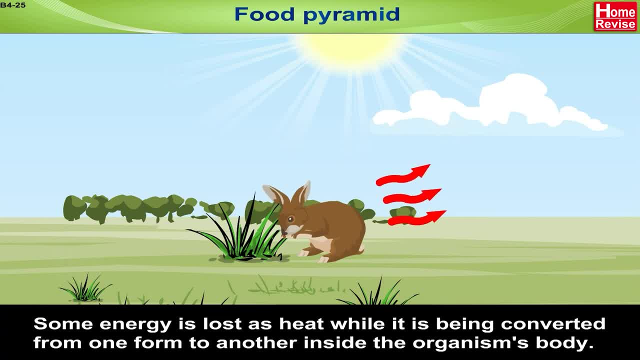 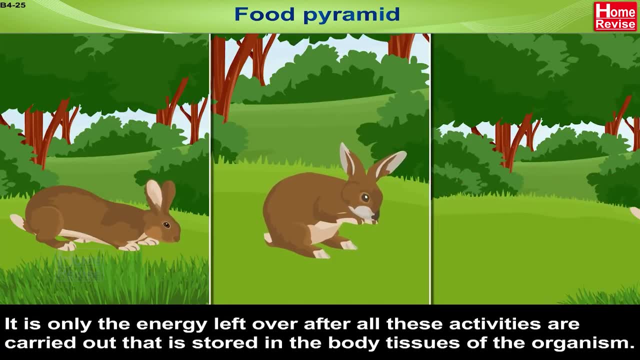 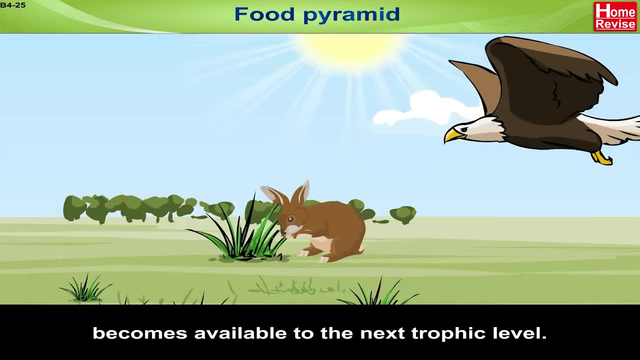 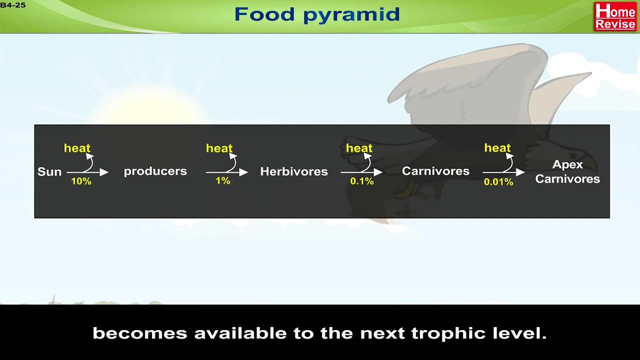 the organism's body. It is only the energy left over after all the activities that have been carried on by the organism. All these activities are carried out. that is stored in the body tissues of the organism and becomes available to the next trophic level. 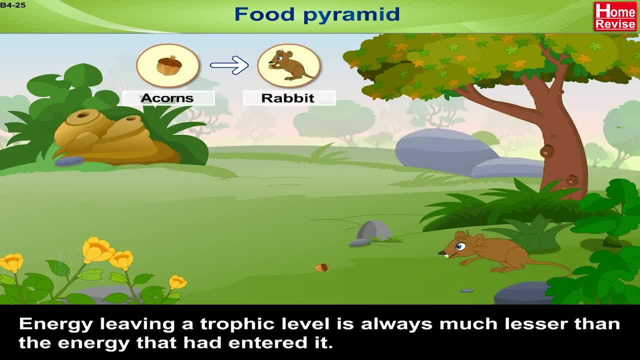 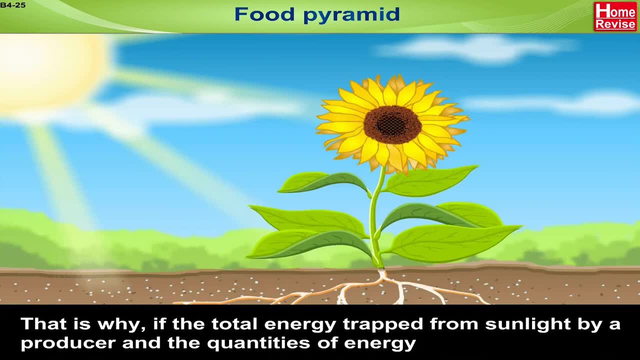 Energy leaving a trophic level is always much lesser than the energy that has entered it. That is why, if you have a trophic level, it is always much less than the energy that has entered it. That is why, if you have a trophic level, it is always much less than the energy that 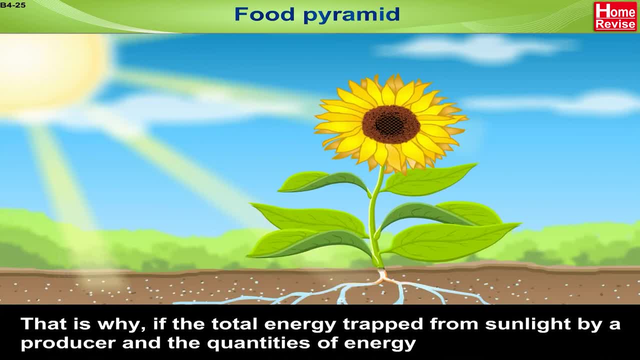 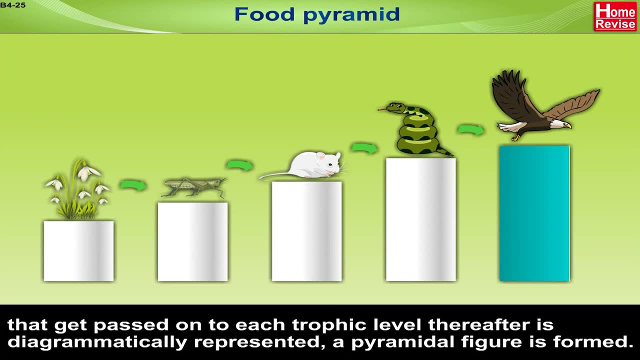 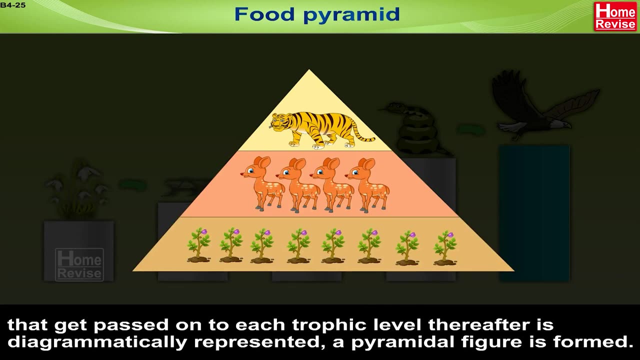 has entered it. With the total energy trapped from sunlight by a producer and the quantities of energy that get passed on to each trophic level thereafter is diagrammatically represented, a pyramidal figure is formed. We call this figure an energy pyramid. 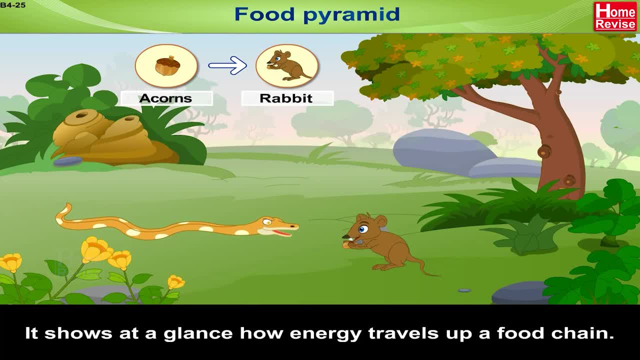 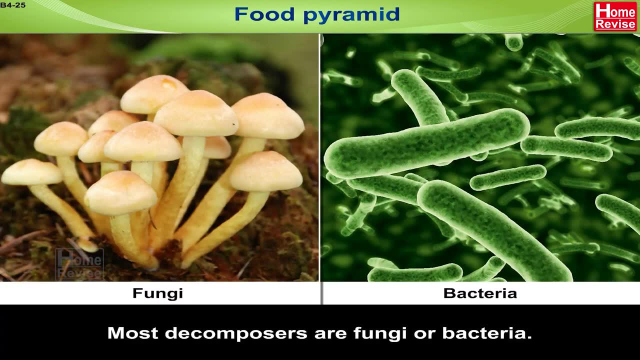 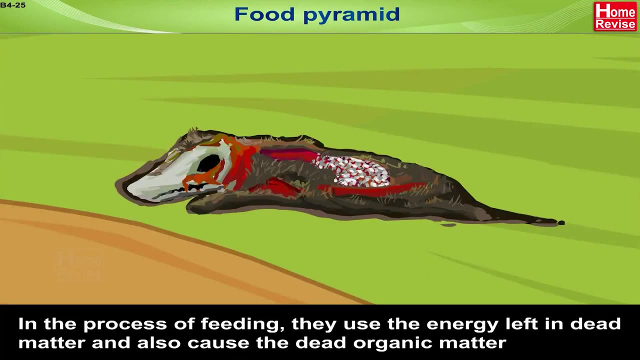 It shows at a glance how energy travels up to the trophic level. In the process of feeding, they use the energy left in dead matter and also cause the dead organic matter to break down into simple substances that easily mix with air, water or soil. 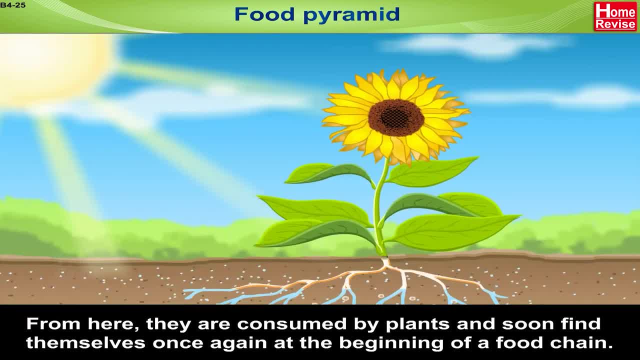 The way that they are decomposed is to make a food chain. They can be made into food grains, so that food grains can be made into meat, meat, vegetables or other type of food. From here they are consumed by plants and soon find themselves once again at the beginning. 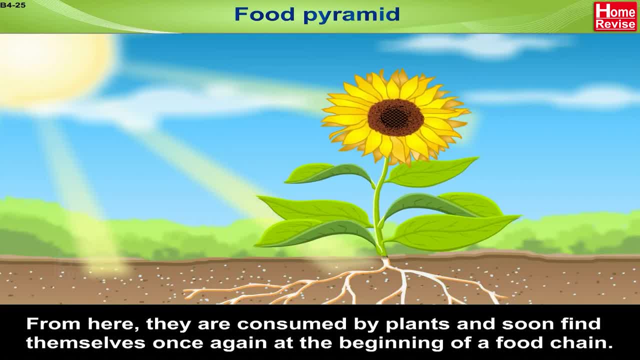 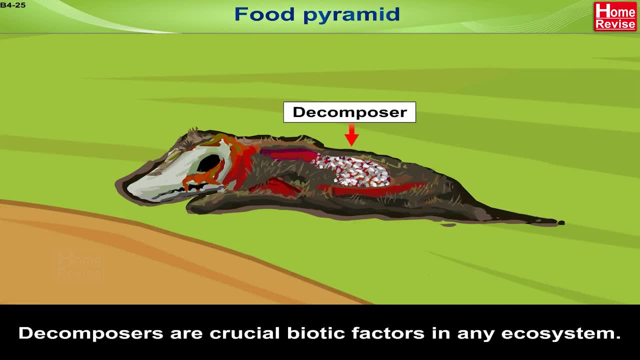 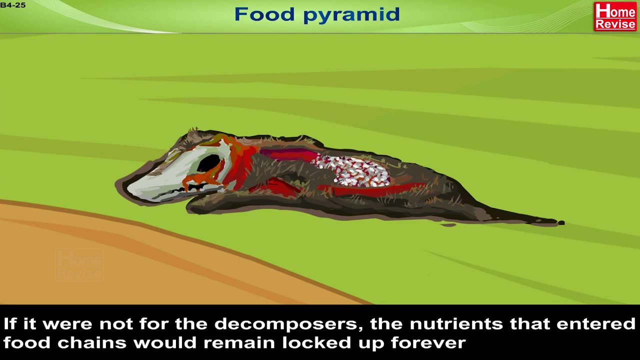 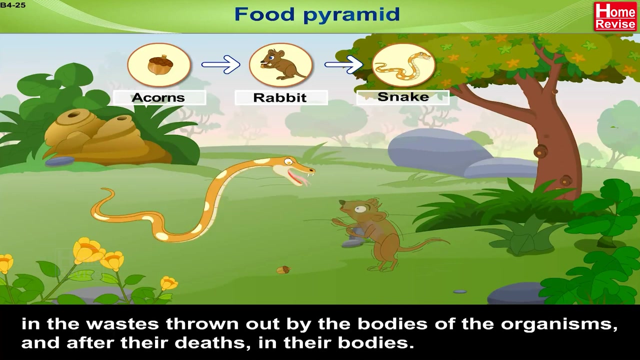 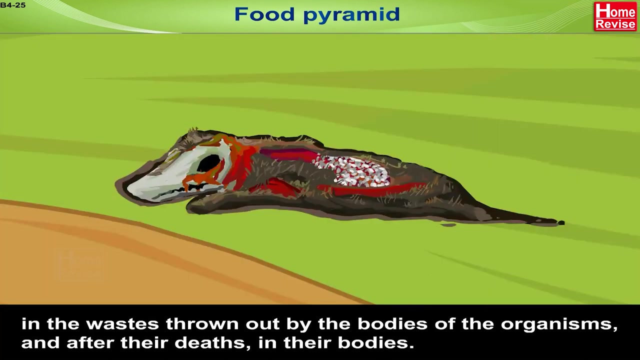 of a food chain. Did you get this till now? Ok, carrying on. Decomposers are crucial biotic factors in an ecosystem. If it were not for the decomposers, the nutrients that entered food chains would remain locked up forever in the waste thrown out by the bodies of the organisms and after their deaths. 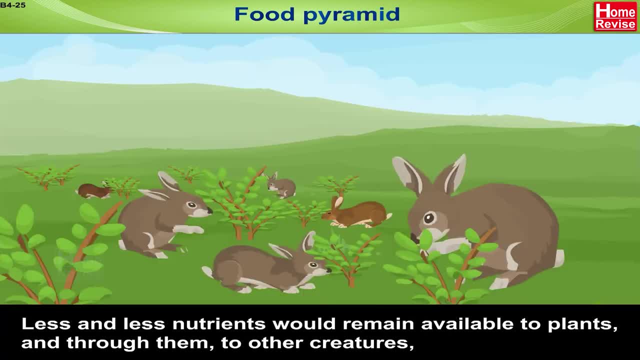 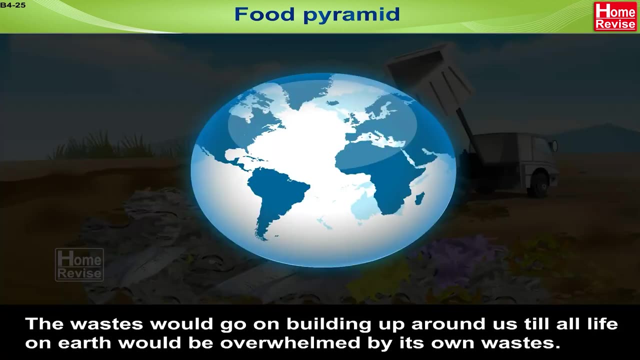 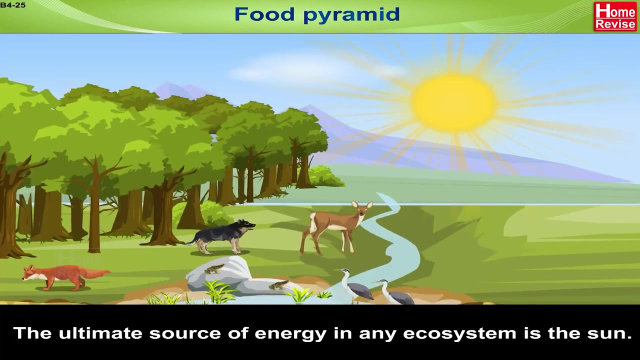 in their bodies. Less and less nutrients would remain available to plants and, through them, to other creatures. The wastes would go on building up around us till all. life on earth would be overwhelmed by its own wastes. But this does not happen, thankfully. The ultimate source of energy in an ecosystem is the sun. 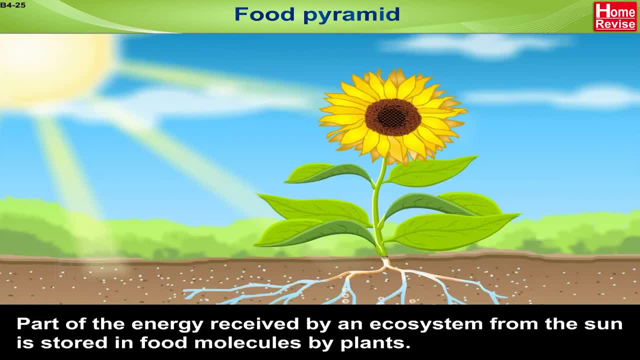 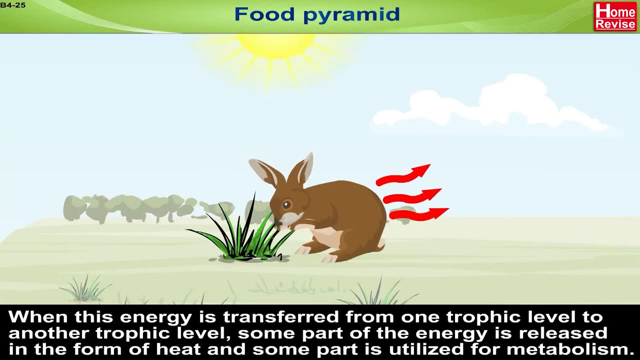 Part of the energy received by an ecosystem from the sun is stored in food chains. This is called a decomposal. The sun is the source of all the energy that is stored in food molecules by plants. When this energy is transferred from one trophic level to another trophic level, some part 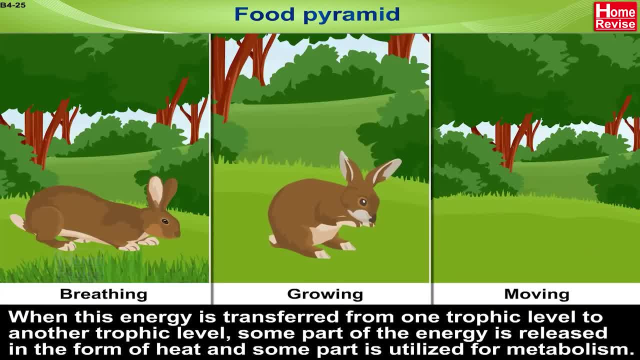 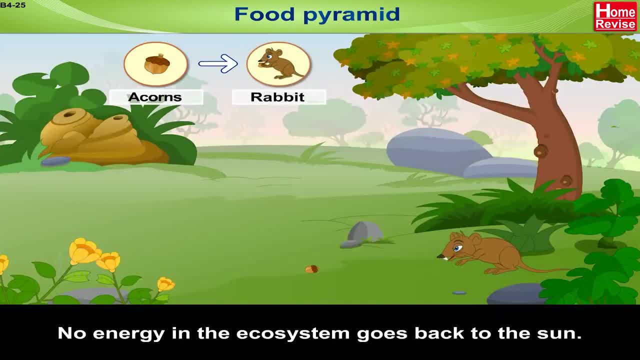 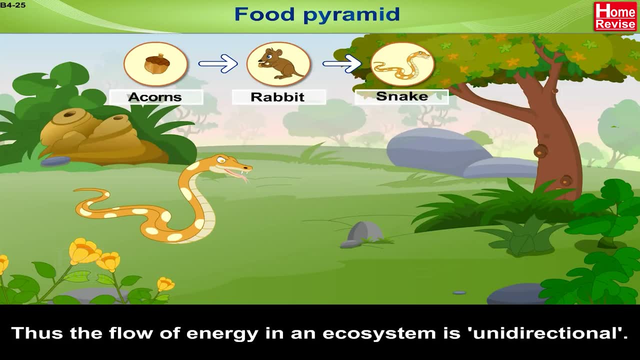 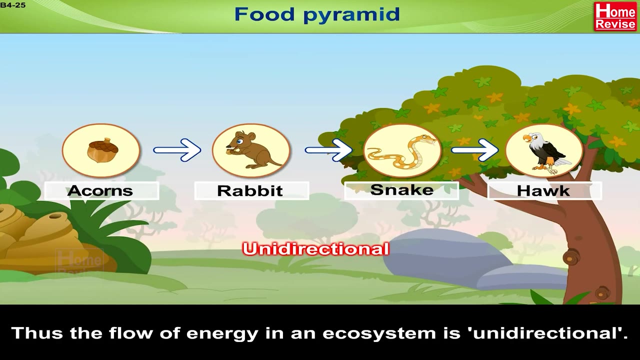 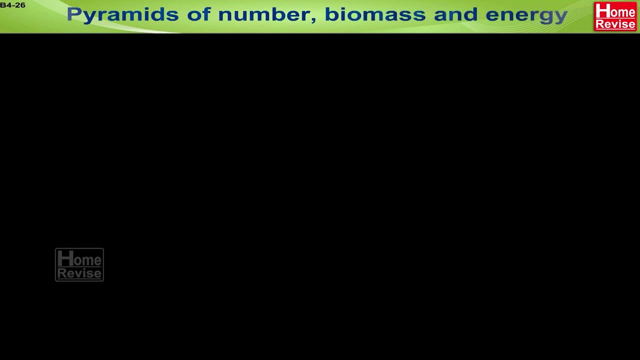 of the energy is released in the form of heat and some part is utilized for metabolism. No energy in the ecosystem goes back to the sun. Thus the flow of energy in an ecosystem is unidirectional. Pyramids of Number, Biomass and Energy.